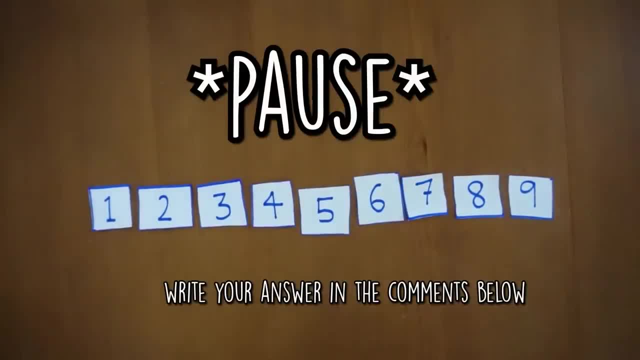 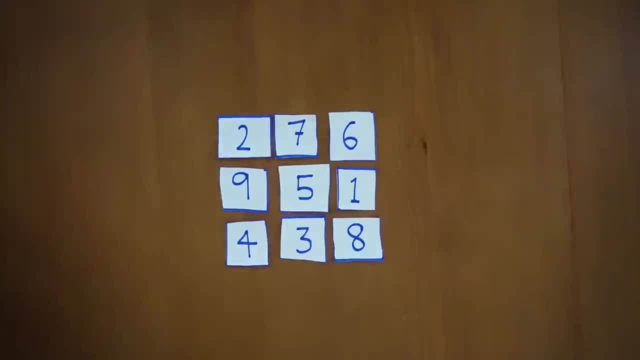 if you'd like to think about it for real, Let me know what you come up with in the comments below. But what if we re-frame the game? instead of lining up the numbers in a line, let's arrange them in a square. These numbers are arranged in a very specific order. 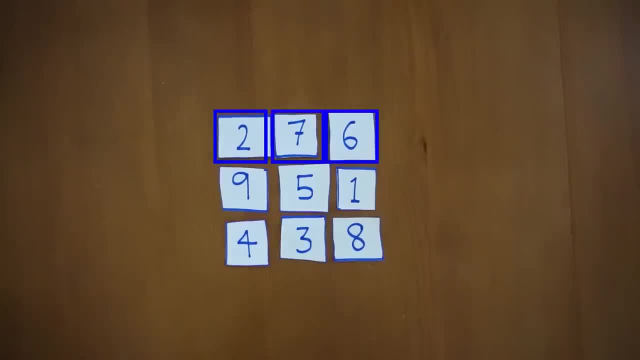 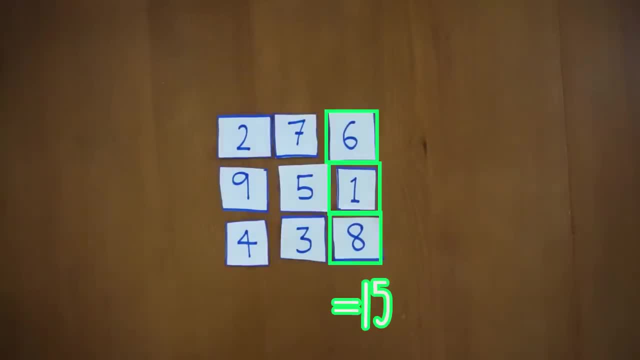 plus five plus four is 15,, six plus one plus eight is 15.. This is called a magic square, where every triplet adds to the same number. Now, how would you try to win the game? It seems more obvious now. You would try to select three numbers which make a triplet. 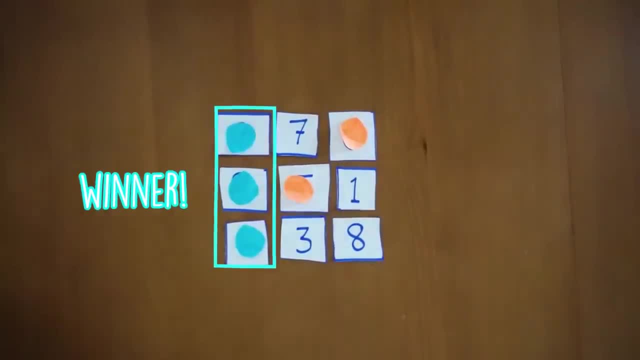 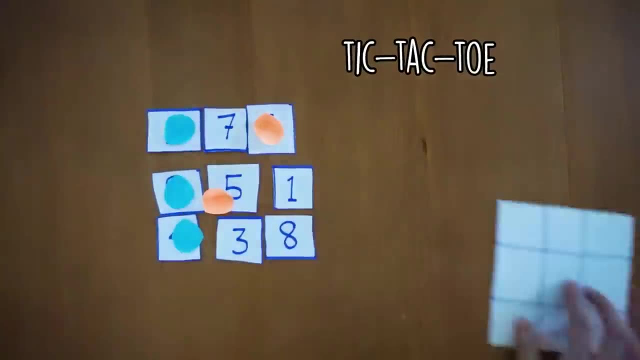 and block your opponent from doing the same thing. Hang on, that sounds oddly familiar. What other game do we know that has those rules? Ah yes, tic-tac-toe, or, as we say in Australia, noughts and crosses. 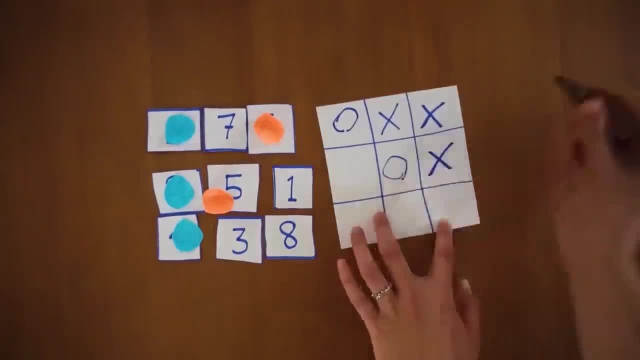 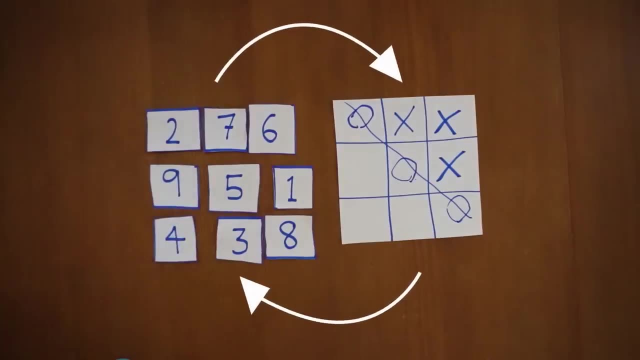 To win, you need to draw three noughts or three crosses in a row, while stopping me from doing that. When we arrange number Scrabble in a magic square, we see it's really the same game as tic-tac-toe. 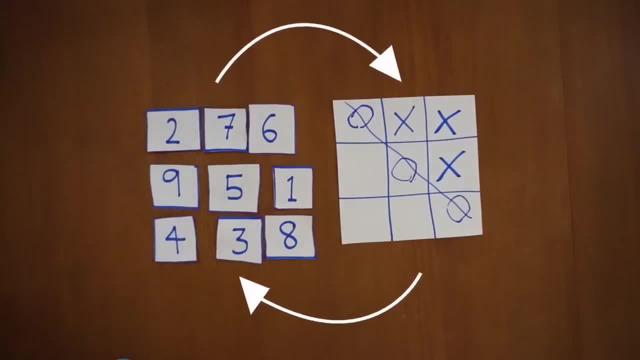 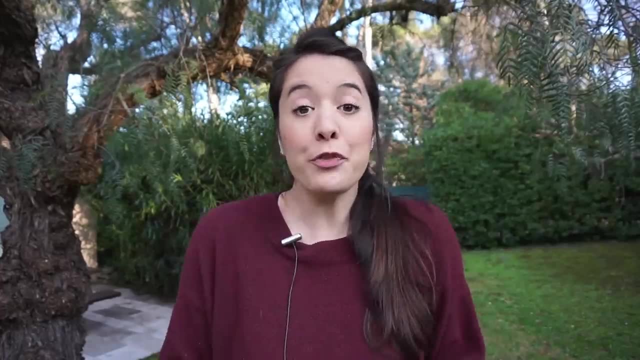 A lot of games can be reduced to the exact same game and a lot of problems in math and computer science can be reduced to the exact same problem. If two problems can be reduced to the same problem, they can be solved by the same strategy. 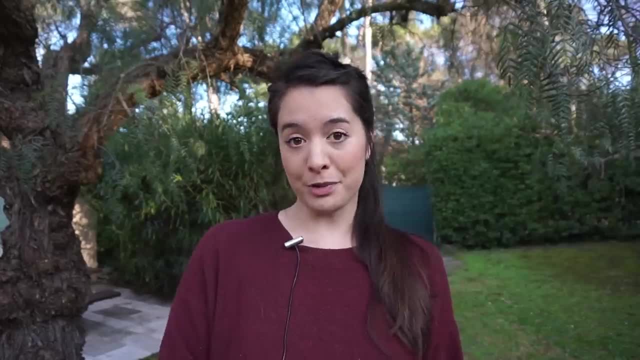 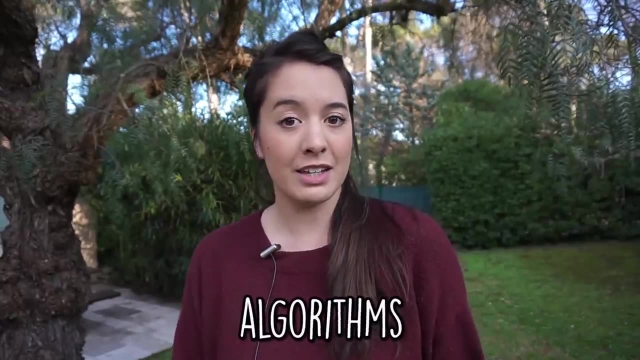 Any strategy that can solve tic-tac-toe can also solve number Scrabble. In math and computer science these strategies are called algorithms and they're mechanical procedures, kind of like a recipe. You don't need to think when carrying it out. 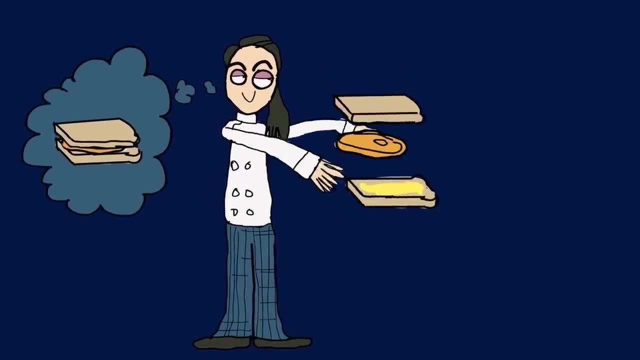 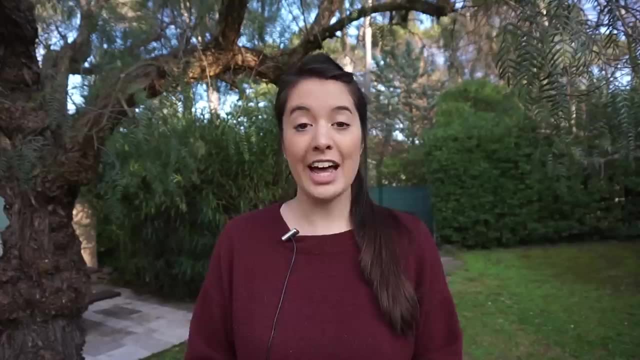 Just follow each step until you reach the solution. Depending on the problem, algorithms can be more or less complex, Just like, depending on the food, recipes can be more or less complex. How complicated an algorithm a problem needs to solve is one of the main areas of interest in computer science. 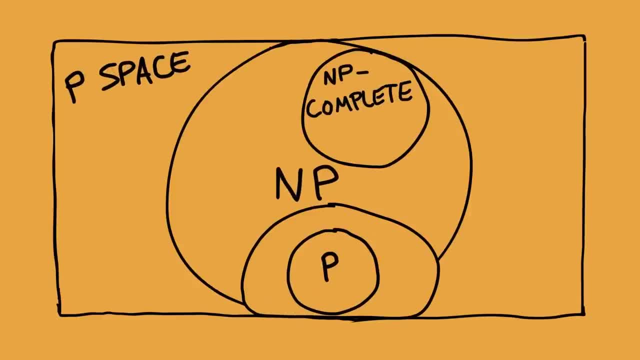 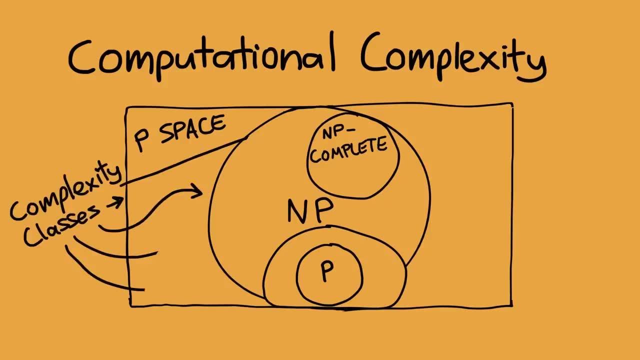 It's so important, in fact, that problems are grouped into classes based on how complicated they are. This area of computer science is called computational complexity, and the groups of problems are called complexity classes. Each complexity class has its own name, and the two we're interested in are P and NP. 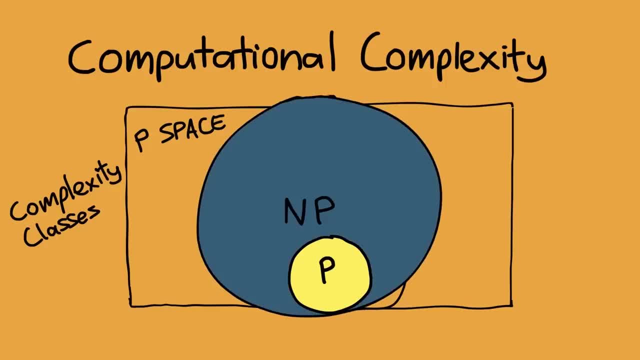 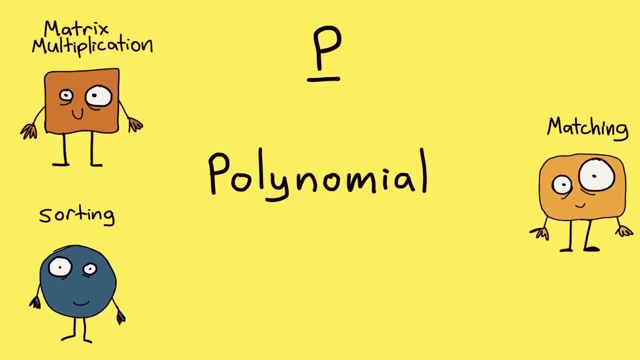 Yes, P and NP are just classes of problems based on how difficult they are to solve. P is the class of all problems which have an algorithm that can be computed in polynomial time. A polynomial is any number that has a power or exponent which is also a number. 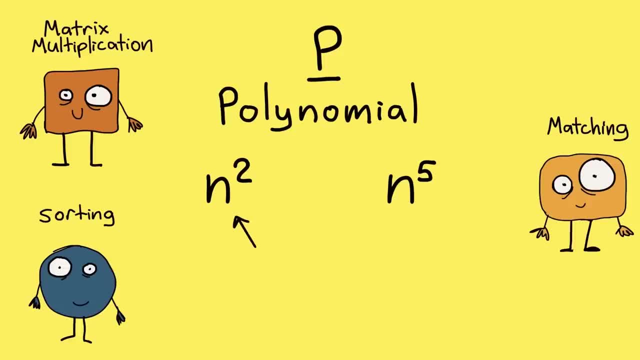 like n to the power of two or n to the power of five. The n refers to the number of inputs to the problem. So we can see that the number of steps the algorithm needs to take is proportional to the input size. This makes sense. 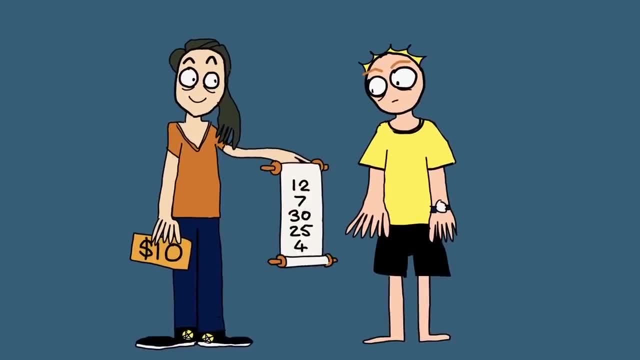 If I asked you to sort this list of five numbers from lowest to highest for $10,, you'd probably do it. But if I asked you to sort this number of 10,000 numbers for $10,, you'd probably tell me to. This is because sorting the larger list takes a lot more steps and so a lot more time. It's exactly the same for computers, except that there are a lot faster than we are and can solve problems with a polynomial number of steps pretty quickly. 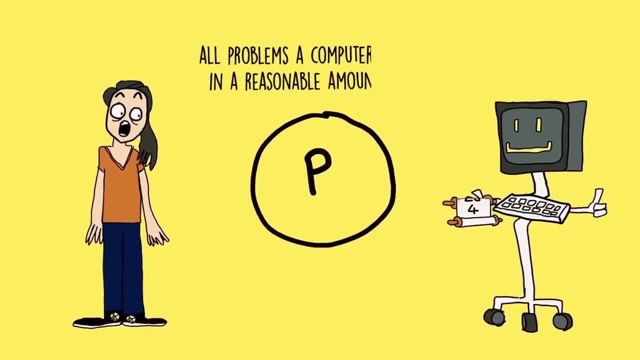 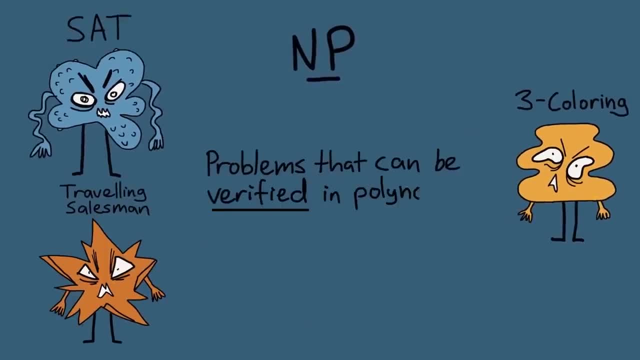 In other words, the class P refers to all problems that a computer can solve in a reasonable amount of time. NP, on the other hand, are the class of problems that can be verified in polynomial time but may take an exponential number of steps to solve. 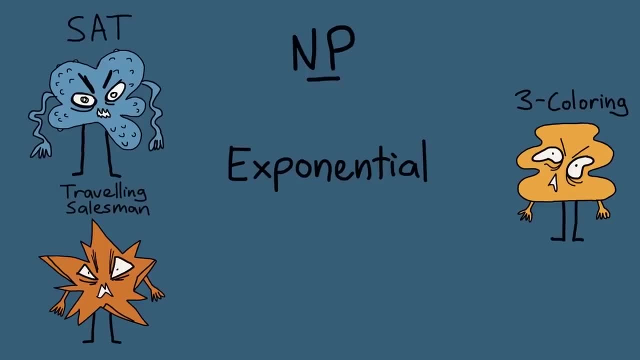 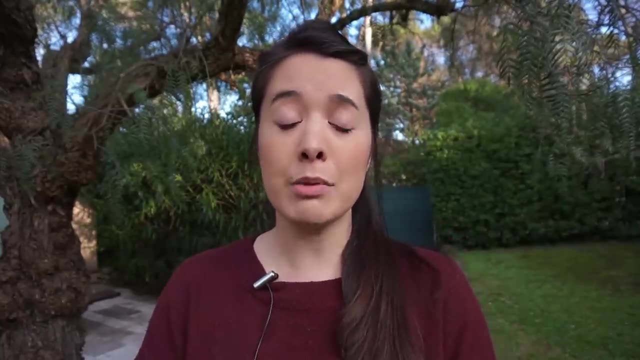 An exponential is when the input number n is in the exponent, or the power like two to the power of n. Now here's the important difference. Computers take a long, long time to solve these kinds of problems. To demonstrate the difference between a P problem and an NP problem. 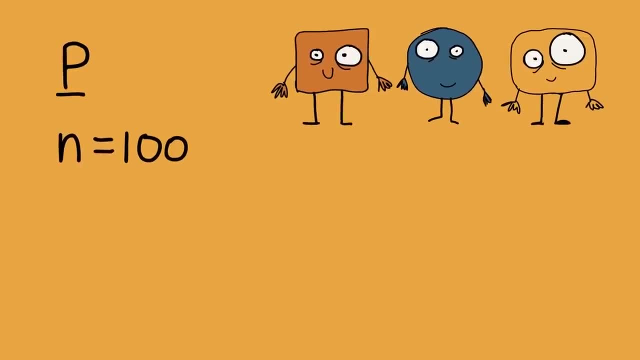 if a problem is in the class P and has 100 inputs and its algorithm is proportional to n to the power of three, a polynomial, it'll solve its problem in about three hours. If it's an NP problem with a completion time proportional to two to the power of n, 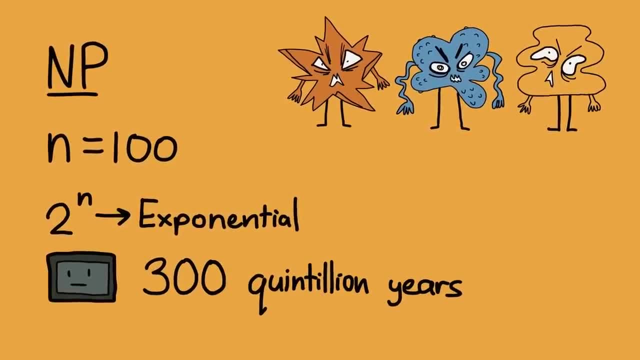 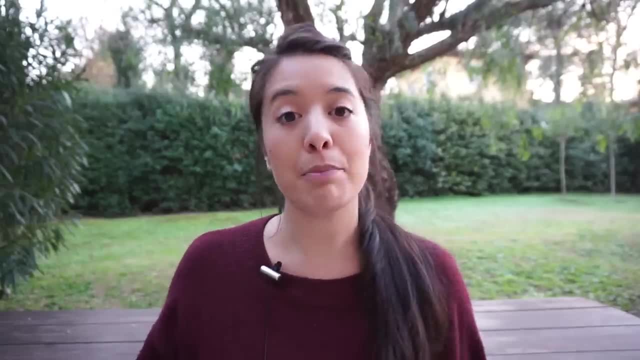 it'll take roughly 300 quintillion years to solve- longer than the age of the universe. So yeah, there's a bit of a difference. but although they take a very long time to calculate, NP problems take a relatively short time to verify. 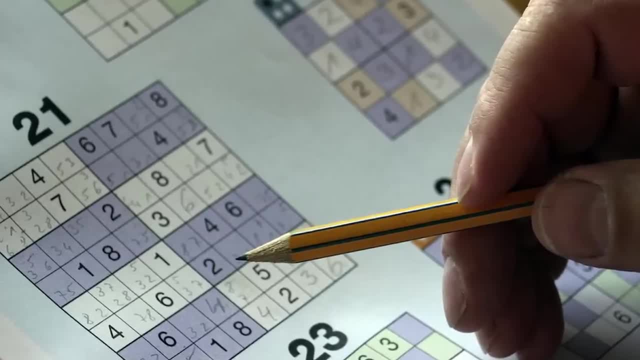 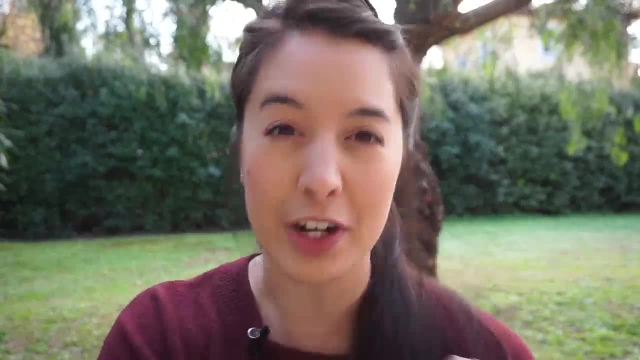 This is pretty intuitive. Sudoku is an NP problem. It takes some effort and time to solve, but once it's solved it's pretty quick to check that it's correct. So now we've finally gotten to the crux of the question. 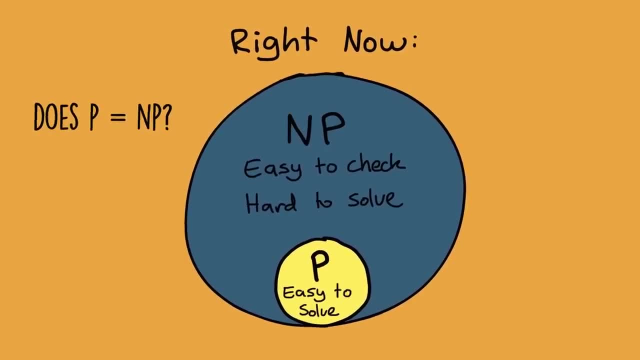 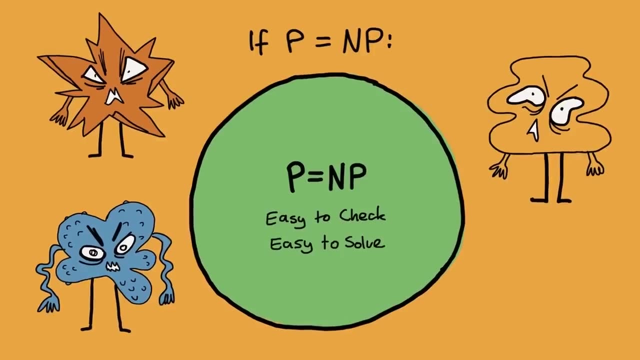 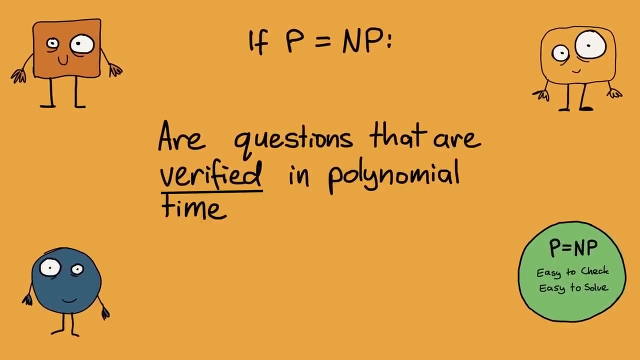 The question: does P equal NP? is asking whether these two complexity classes, P and NP, are in fact the same class. That is, can we perhaps solve these exponential problems in polynomial time? Or, framed another way, are questions that are verified in polynomial time? 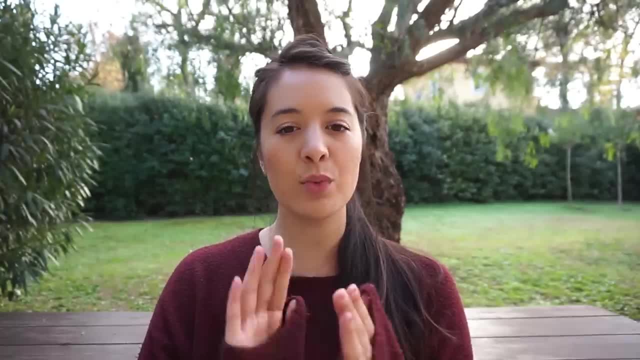 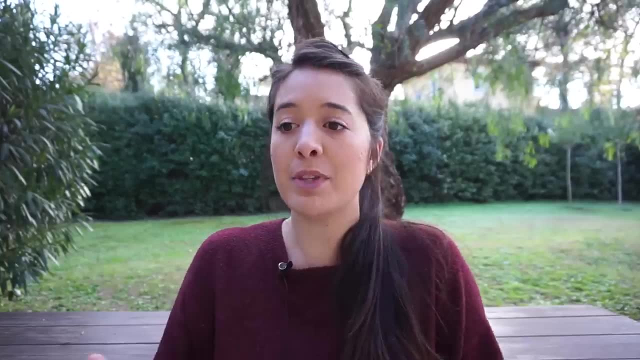 also solved in polynomial time. Now, it was at this stage in my research that I found something deeply confusing, and that is why is this even a question, I mean for something to be called the biggest open problem in computer science. there needs to be some kind of ambiguity. 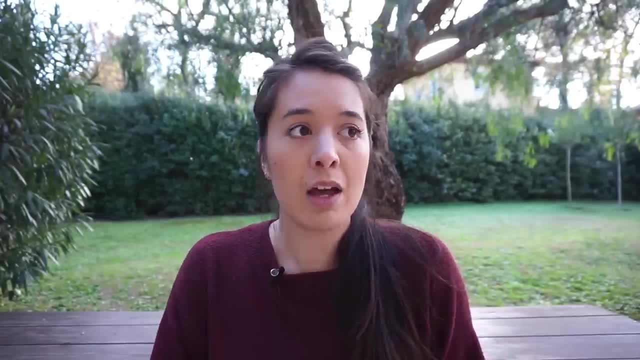 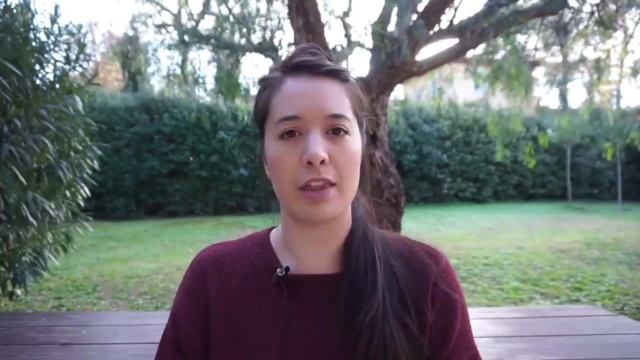 around the answer right Like: do we have any reason to believe that P might equal NP? I mean, the question is basically asking: is this thing that doesn't look like this other thing really that thing? This annoyed me so much. 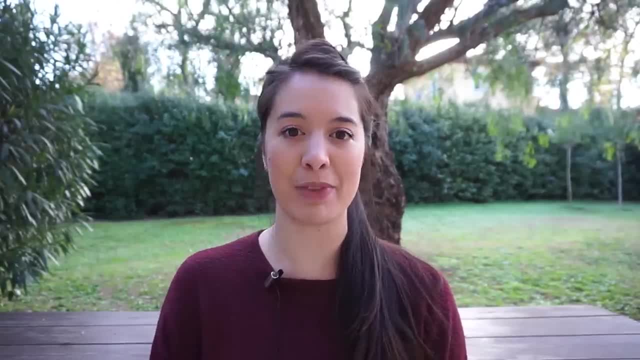 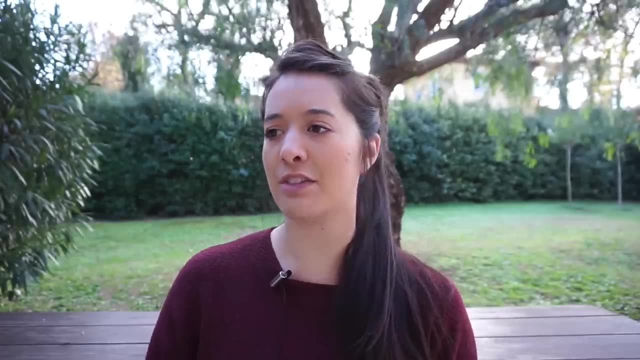 that I spent two whole afternoons Googling it and I found three things. One: most computer science researchers don't think that P equals NP, Okay, Two: a somewhat unsatisfying answer to my question was that well, it hasn't been proven. 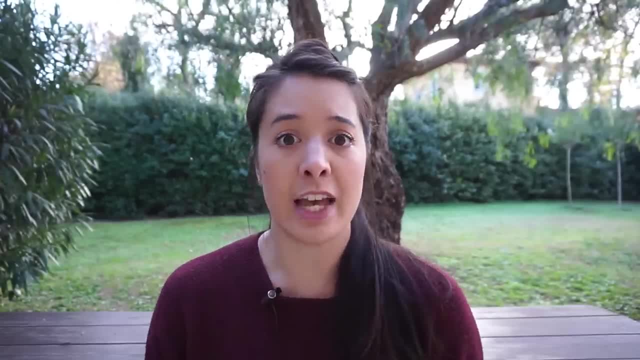 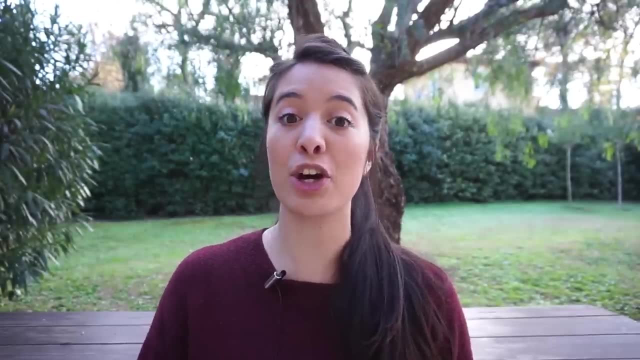 that P doesn't equal NP. but I mean, a lot of things haven't been proven. It hasn't been proven that you can't raise people from the dead and there's no million dollar prize about that. And three, another common reason. 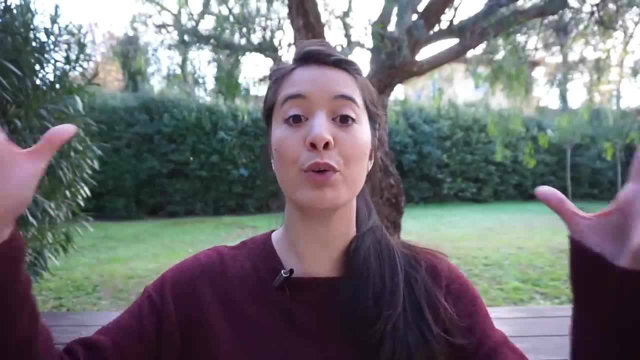 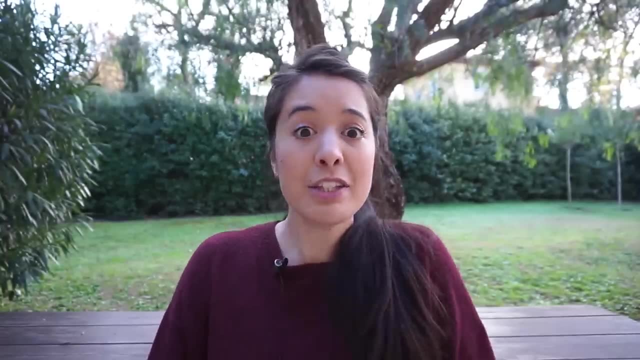 I came across for why this is a question is that it would improve the world by unimaginable amounts. if unimaginable amounts, if P did equal NP, But I mean lots of things would improve the world a lot Like. why is this question a question? 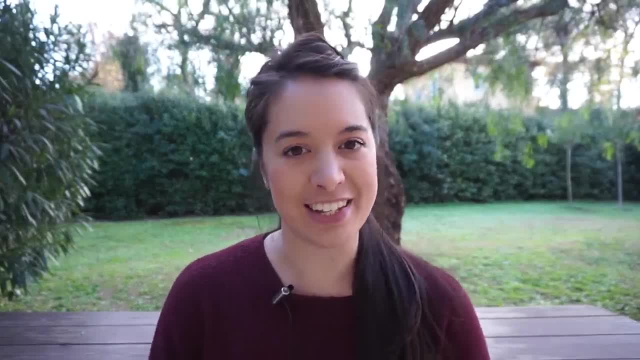 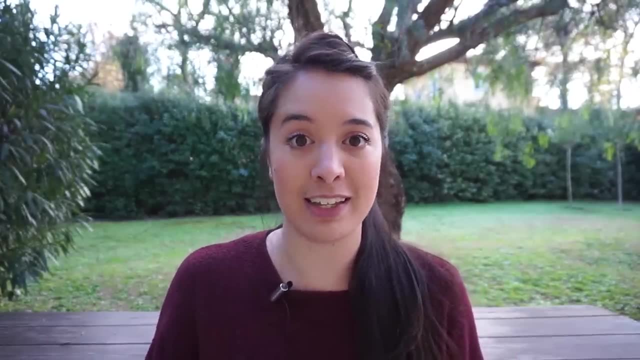 At the end of the afternoon I did come across what I found to be a reasonable answer. But before I tell you that, I'd first like to tell you what would happen if it turned out that P did equal NP Optimization problems like transport routing. 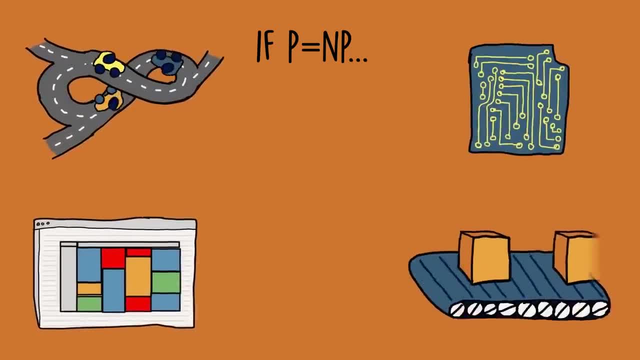 production of goods, job scheduling, circuit and database design are all NP problems. Imagine how much more efficient the economy would be if we could find the most optimal solutions to all these problems. There would be massive advances in machine learning as problems that are easy to check. 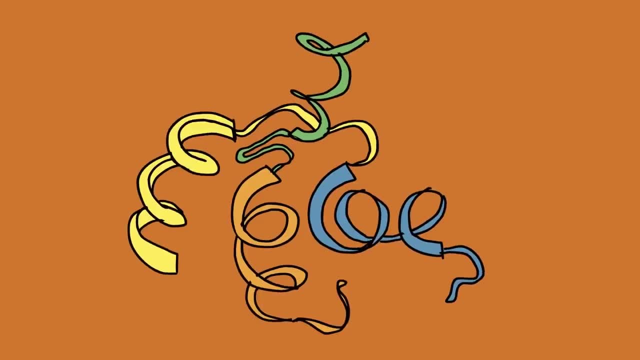 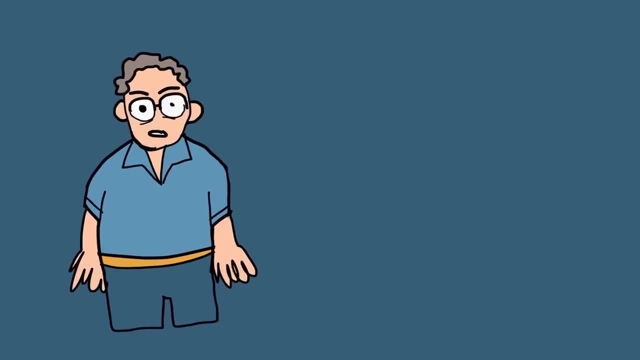 would become just as easy to solve. The problem of protein folding is an NP problem. If we could solve it, we could cure cancer. To quote MIT complexity researcher Scott Aronson, if P were equal to NP, then the world would be a profoundly different place. 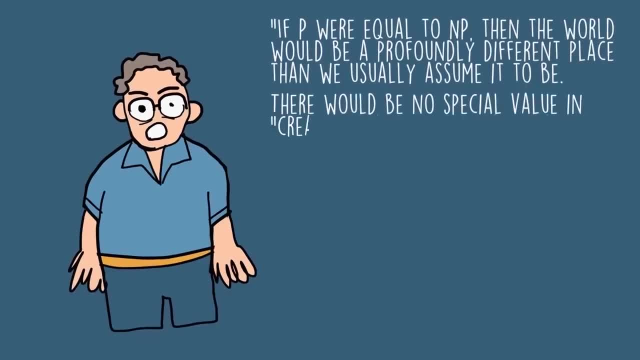 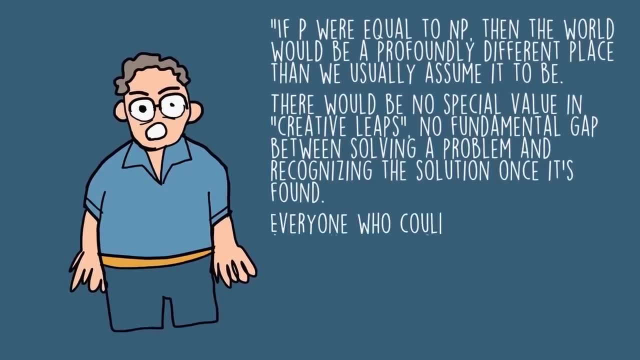 than we usually assume it to be. There would be no special value in creative leaps, no fundamental gap between solving a problem and recognizing the solution once it's found. Everyone who could appreciate a symphony would be Mozart. Everyone who could follow a step-by-step argument. 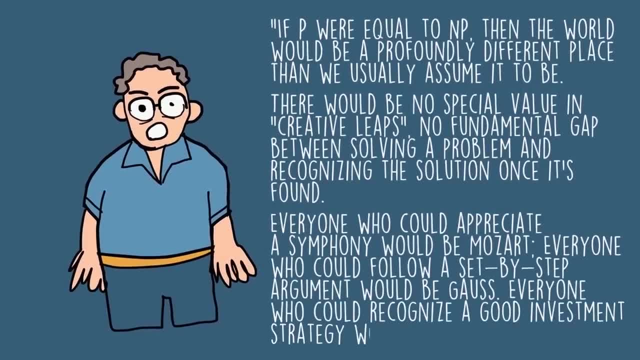 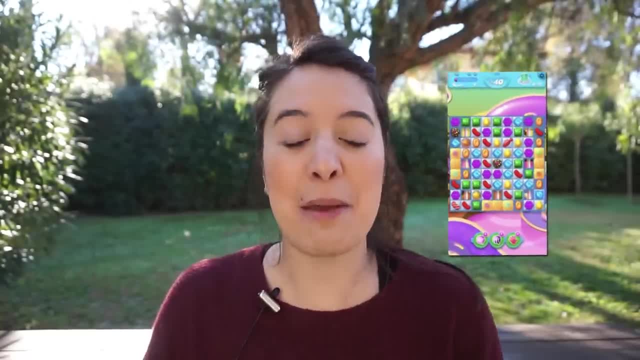 would be Gauss. Everyone who could recognize a good investment strategy would be Warren Buffett And, most importantly, we could finally be Candy Crush. Yes, Candy Crush is one of these NP-highlights. It's hard to find a solution to these hard problems. 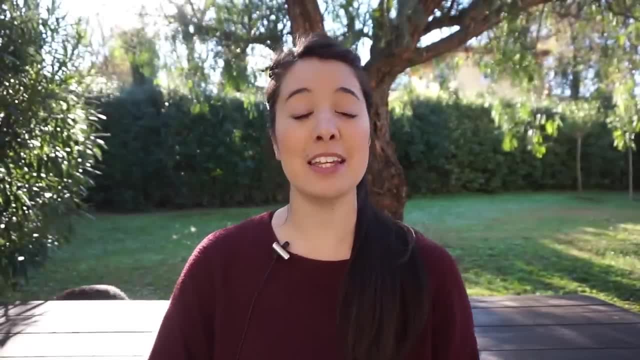 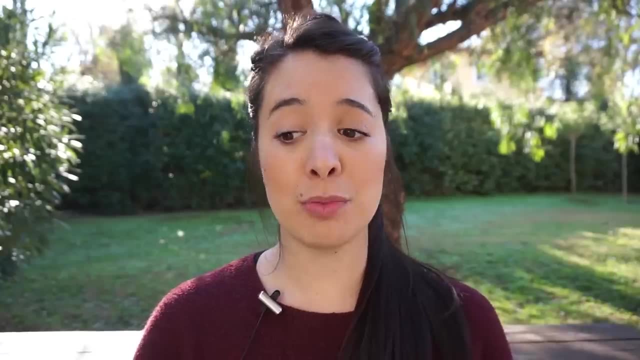 However, there is a downside to this golden metropolis: Encryption. the math that keeps your bank details and privacy safe relies on P being different to NP. If P were shown to be equal to NP, all of your passwords and therefore all of your information. would be free game for the world. So, apart from you potentially losing your life savings, it'd be pretty cool if P did equal NP. Being able to solve any problem, as checking the solution to that problem would make life insanely easier. There's no lack of motivation for wanting P to equal NP. 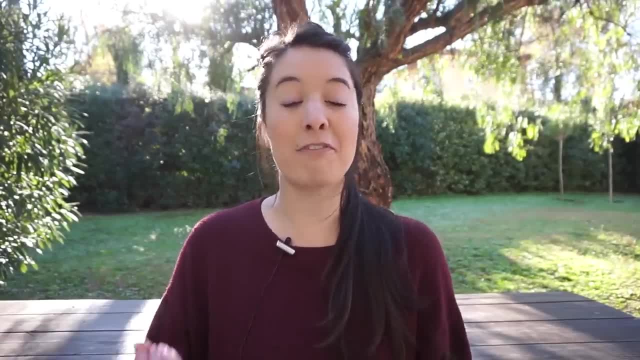 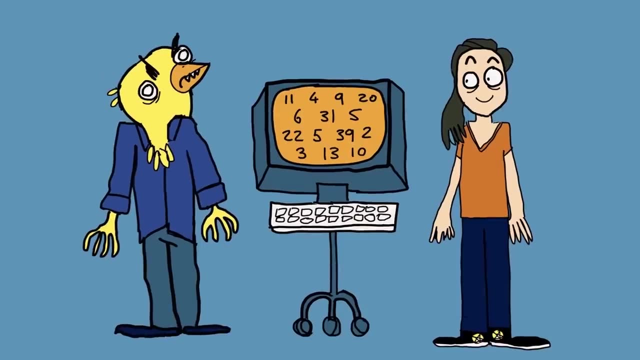 But just because it would be nice. why does that mean it's a major and famous problem in computer science. Well, to understand that first, imagine this scenario: Your boss asks you to sort this list of numbers. You've fluffed your way through the job interview. 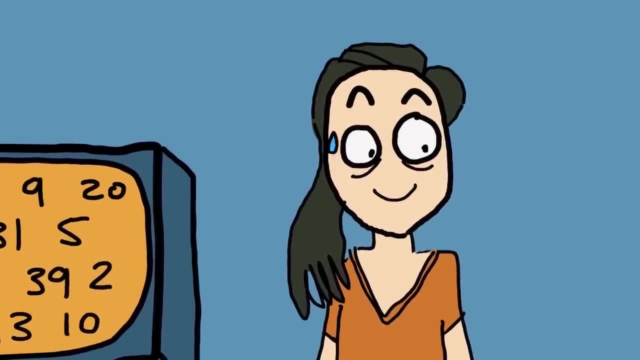 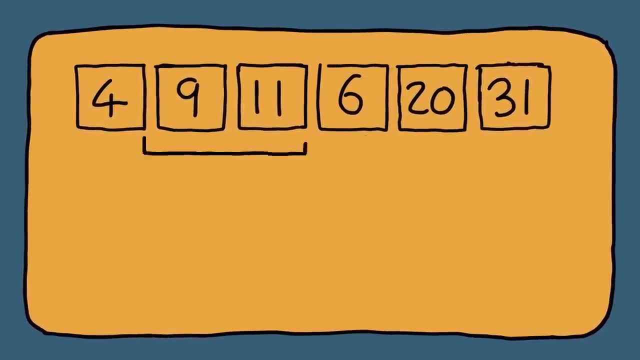 and don't know much about coding. so you write a very simple algorithm. It goes through an entire array and compares each neighboring number: The larger value on the right and the smaller value on the left. It continues this process until the array is fully sorted. 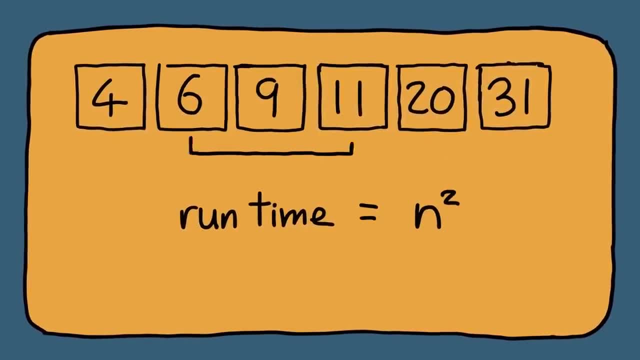 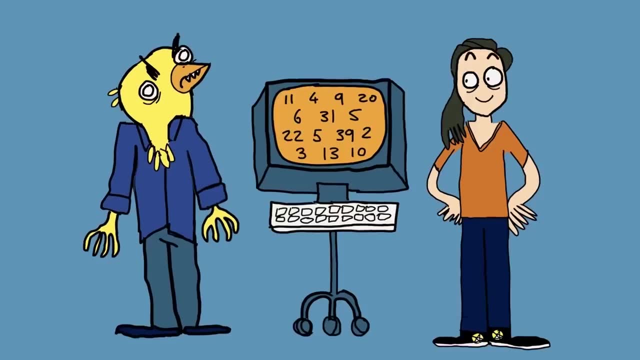 The runtime of this algorithm is of the order of N to the power of two, which means that if there are 100 inputs, it will take a maximum of about 10,000 steps. You're pretty proud of yourself, but your boss isn't happy. 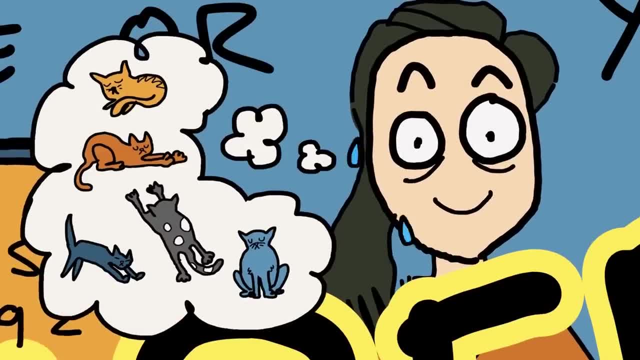 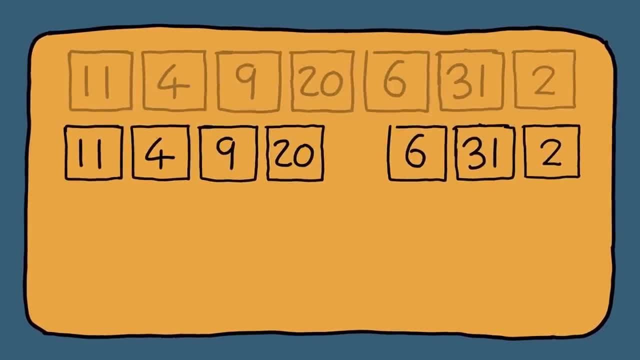 Make a faster one or you're fired. You've got a family to feed. You've got to get serious. You write a new program which takes an array, splits it in two down the line, splits it down the middle and keeps doing so until there are only squares of one left. 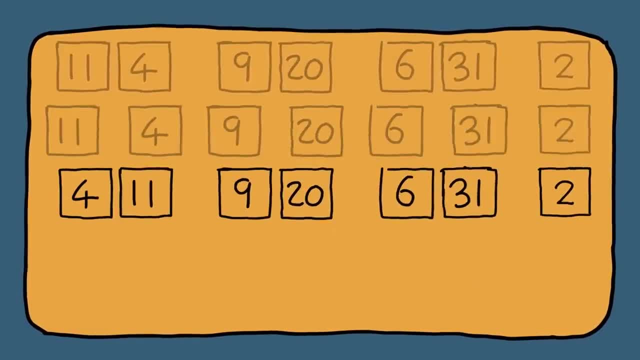 It takes two neighboring squares and sorts them with the lower number on the left and the higher number on the right. It then looks at the neighboring pairs and compares the lower numbers with each other, sorts them, then compares the higher numbers and sorts them. 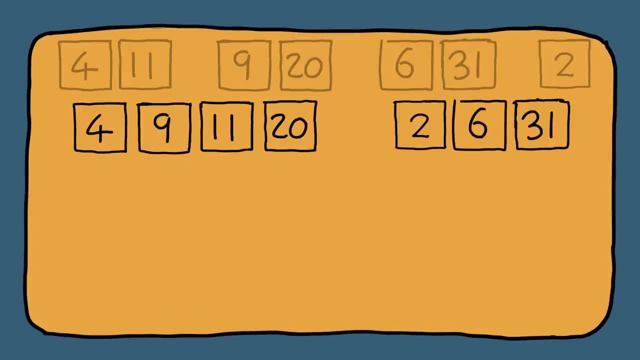 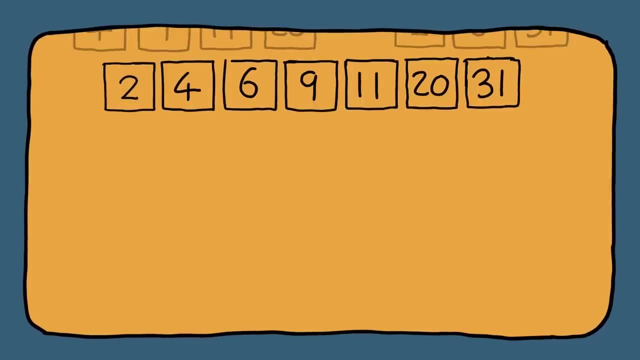 then combines the array. It keeps repeating this process, which in turn takes the two arrays and compares the values of the first number of each array, Comparing and sorting like squares, and then combining everything until finally we end up with a full array of sorted numbers. 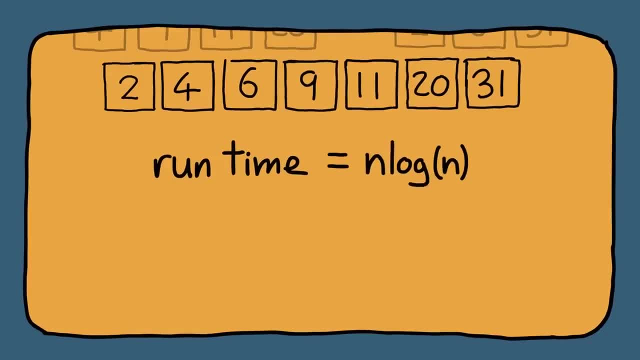 This new algorithm has a runtime of the order of n log n, which means that if there are 100 inputs, it'll take around just 200 steps- a massive improvement on the 10,000 steps from before. It looks like you deserve the job after all. 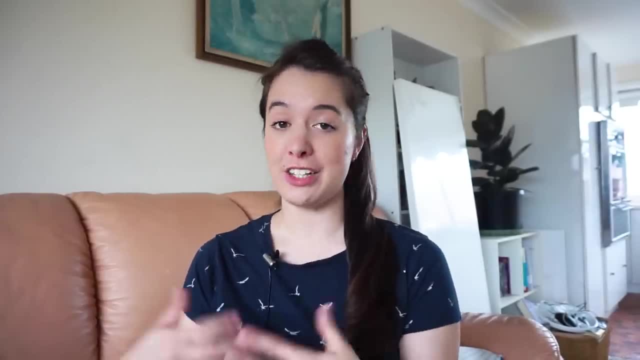 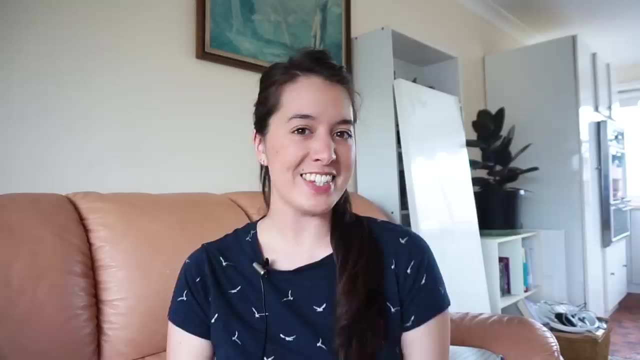 The point of all of this is is that sometimes you can improve an algorithm so that it solves a problem faster. The problem didn't change. You still needed to sort it. You still needed to sort a list of numbers, But by being clever and a bit scared. 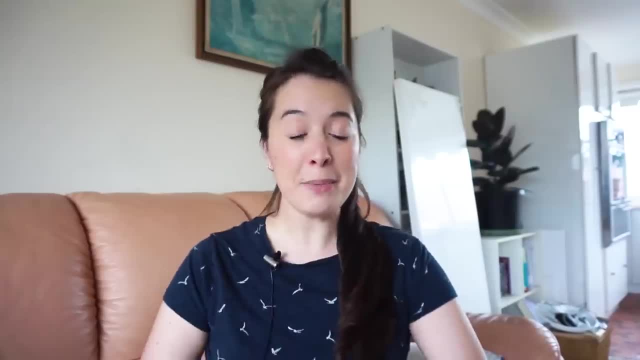 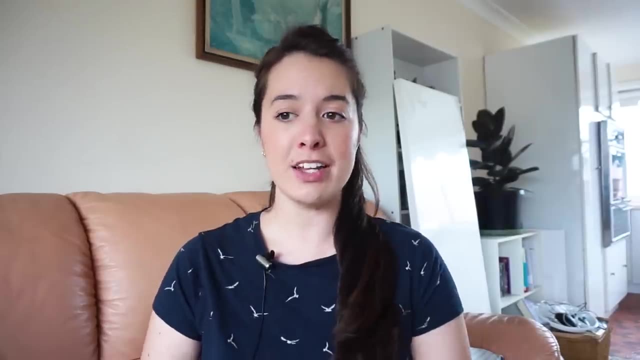 you managed to find a faster way to do it. This is exactly what happened in the case of some NP problems. It was deemed that they couldn't be solved in polynomial time, but then some clever person came along with an amazing algorithm and managed to transport the problem from the NP realm. 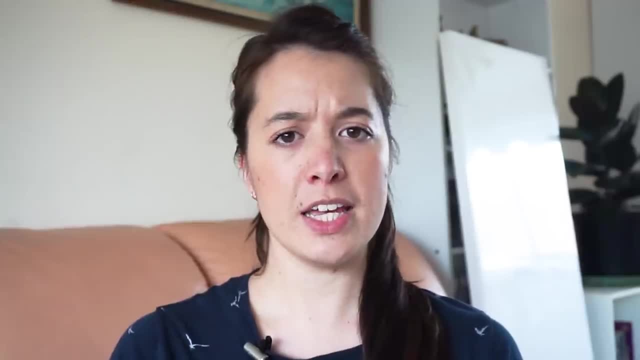 to the cozy-comfiness of the P realm. Now you're probably thinking: wait, Jade, if it was shown that some NP problems were in fact equal to P, doesn't that prove that? you know, some NP problems were in fact equal to P? 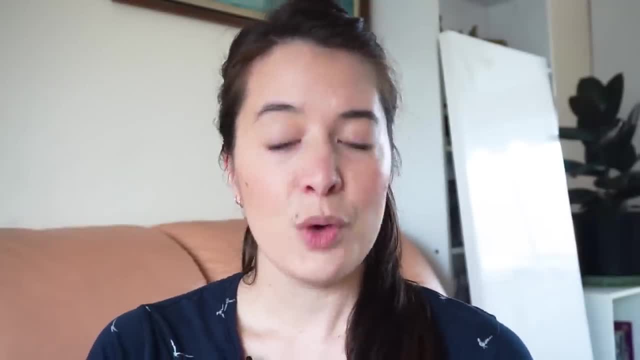 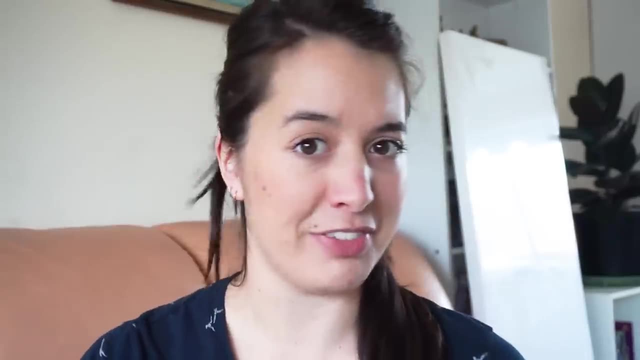 Doesn't that prove that, you know, P equals NP? Well, you would think so, but the answer is no. Here's where things get a little bit fiddly, but just pay attention and you'll be fine. So complexity classes aren't like totally separate things. 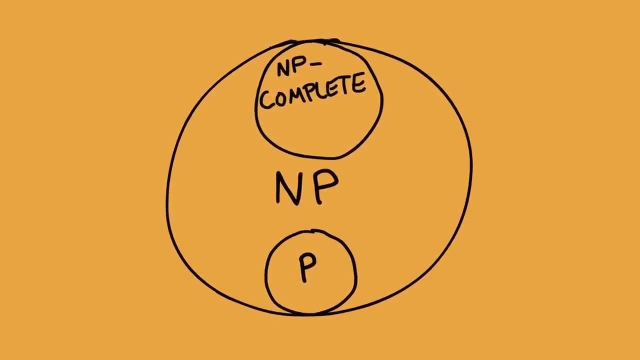 Some of them are more like Russian dolls in that they contain other classes. You'll see that the class of P is actually contained within NP. See, not all problems in NP take the same amount of time to solve, but rather they can all be solved. 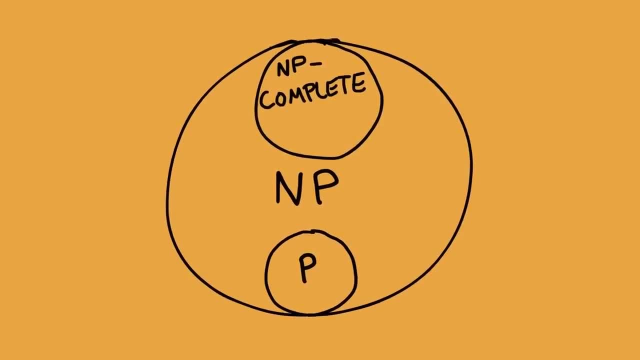 in exponential time or less. Problems in P can obviously be solved in exponential time or less. If you can solve something in less than a hundred years, you can definitely solve it in less than a thousand years. So NP is the class of all problems. 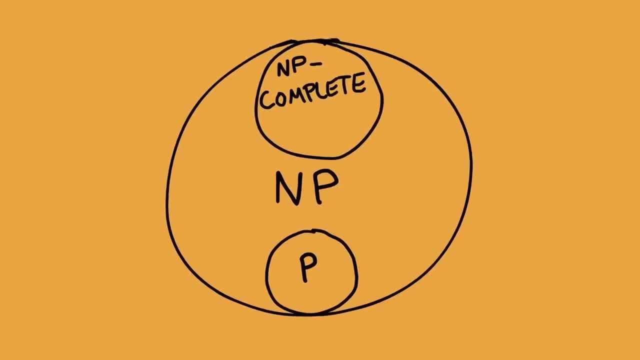 that can be solved in exponential time or less. Now see this NP complete circle here. They are the hardest problems in the whole class of NP and they take the longest time to solve. Some problems from the middle of NP were shown to be in P. 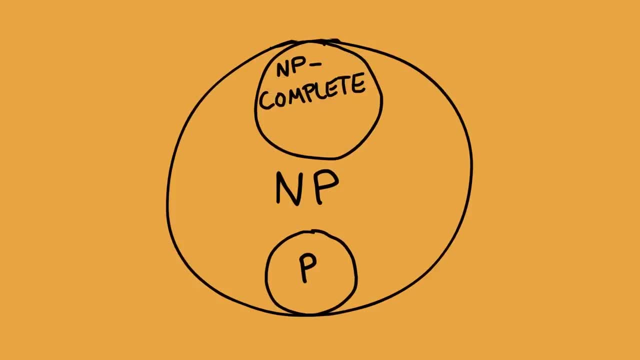 but none of the NP complete circles were solved in NP. Some problems from the middle of NP were shown to be in P, but none of the NP complete problems ever have been. So the question: does P equal NP really means? are NP complete problems the hardest problems in NP in the class P? 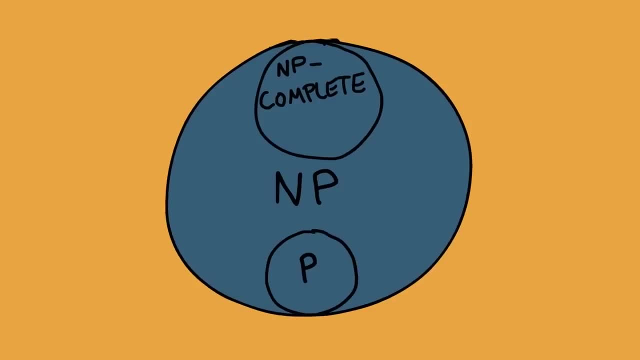 Was that confusing? I got a bit confused. Let me say it again: NP problems can all be solved in exponential time or less. Some NP problems, those in P, can be solved in polynomial time or less. Therefore, the class P is contained within NP. 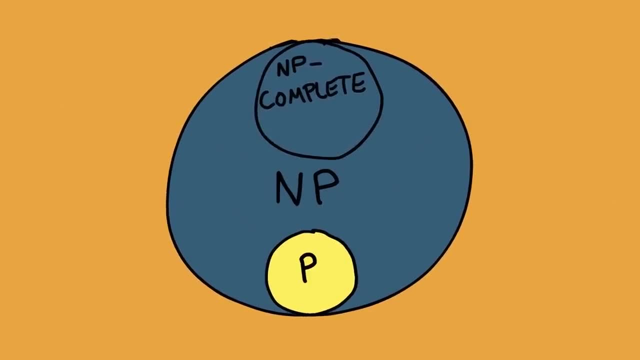 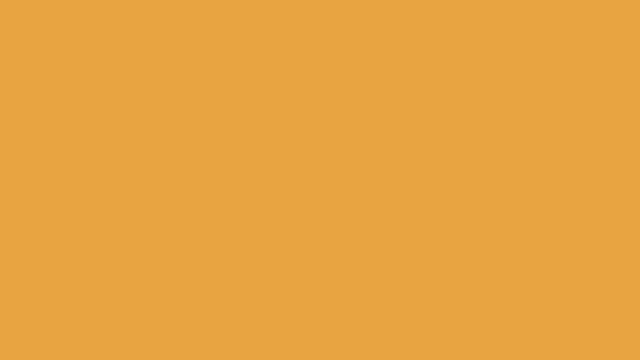 NP problems have been shown to be in the class P. However, the hardest problems in NP, the NP complete ones, have never been shown to be in the class P. So the question of whether P equals NP still isn't solved, because this NP refers to NP complete problems. 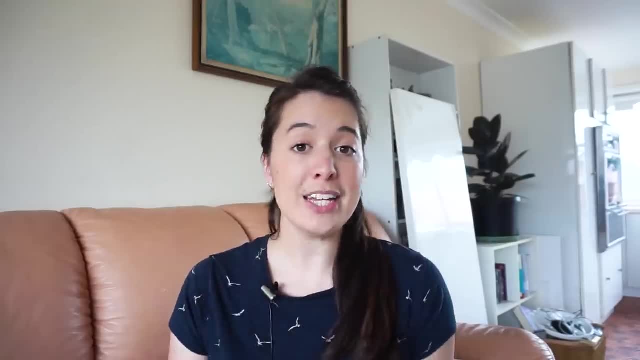 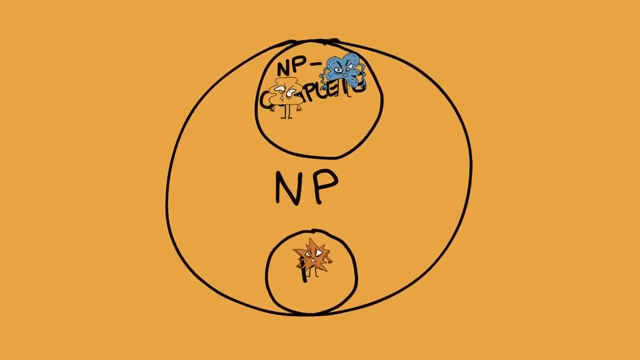 And now to return to the original motivation for this whole bit: Why is P equal NP- such a big question? Well, if just one of the NP complete problems was shown to be in the class P, that would mean that all of the NP complete problems. 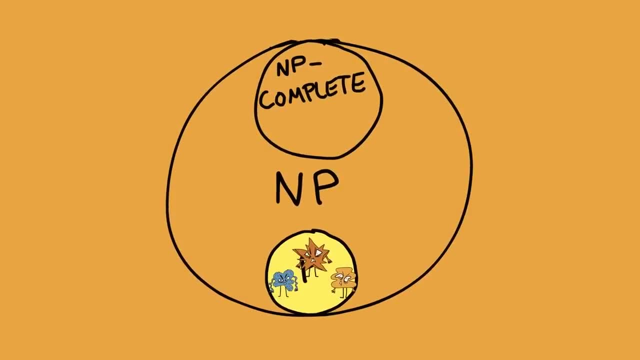 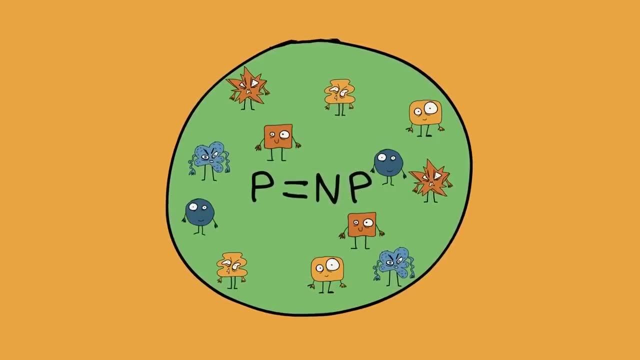 would be in the class of P. Just like solving number Scrabble also solves tic-tac-toe, And if some NP problems have been shown to be in P, it's not too crazy to think that maybe just one NP complete problem might be in the class of P. Maybe some rebel with a totally radical idea will come up with an amazing algorithm. If they showed that just one NP problem could be reduced to a P problem, this would show that all NP problems could be reduced to P problems and that P does in fact equal NP. 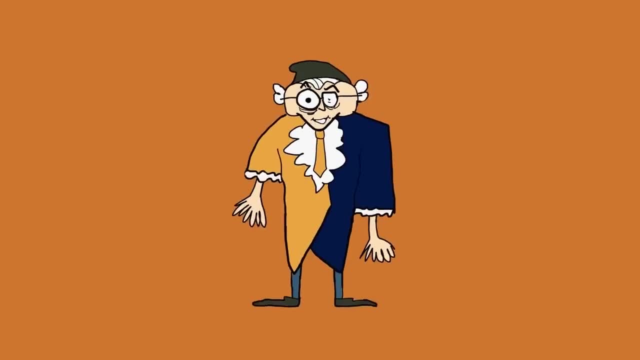 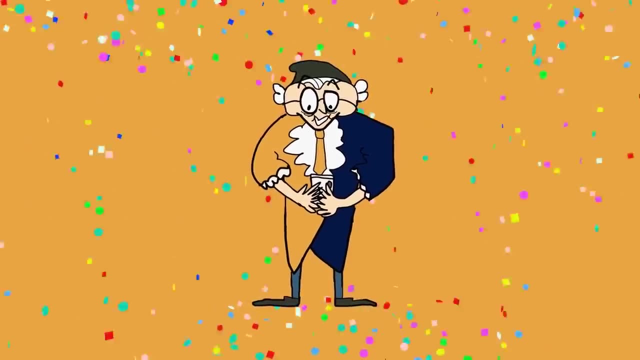 You could be Mozart, Warren Buffett and Gauss all in one. Cancer would be cured and you could finally get to work on time And, most importantly, beat the high score in Candy Crush. We've seen today that a powerful algorithm has the potential to change your life for the better. 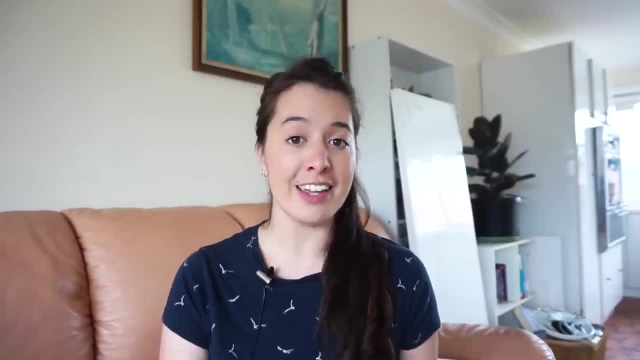 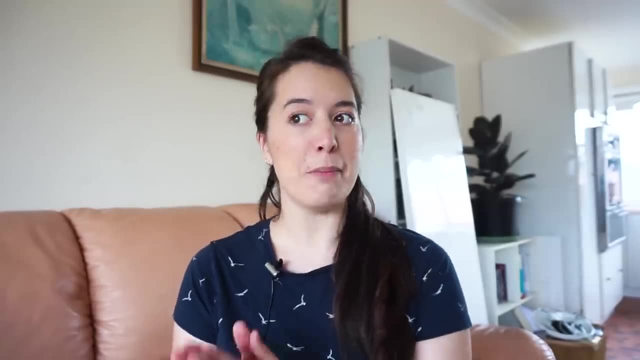 But what powerful algorithms already exist that you can start using today. For example, did you know that there was an algorithm that will tell you the best strategy to try new things? There's an algorithm that tells you when the best time to try new things is. 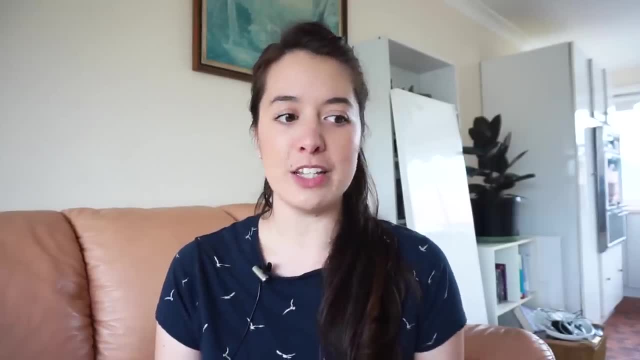 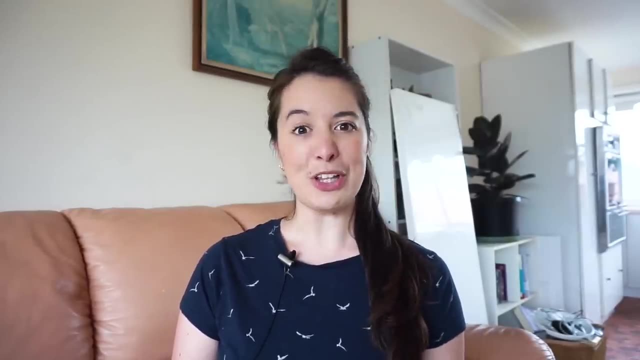 and when to stick to what you know. Another one to tell you when to reconnect with friends and when to leave things to chance. When I first started getting interested in computer science, what fascinated me most was the pure logic behind it, how you can take a very abstract question. 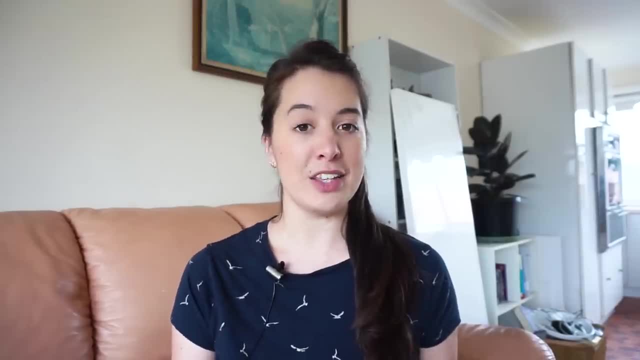 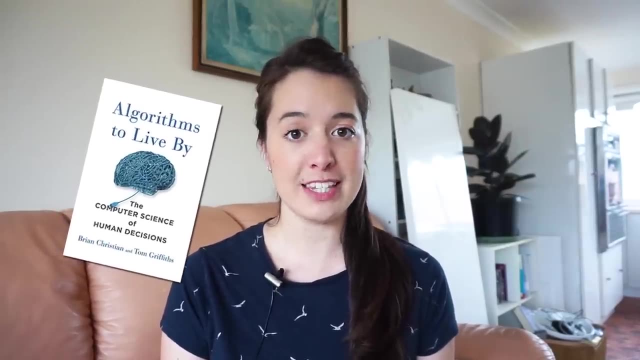 like: when should you try new things and break it down and even come up with an algorithm to solve it? One of the first books I read was Algorithms to Live By, and it was a very interesting book. It's written in a very nice conversational tone.